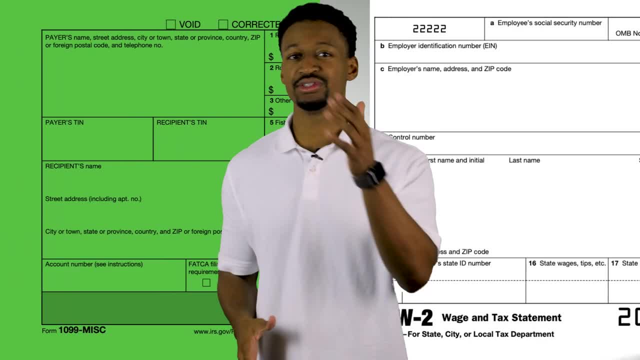 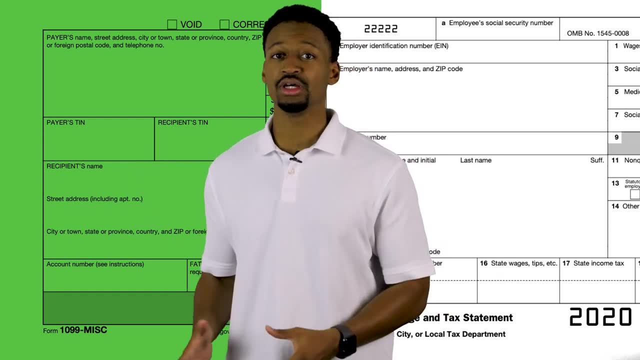 In other words, we're going to debate whether you should use a 1099 versus a W-2 and which one may be best for your business, Because selecting between these two will determine your tax outcomes, for both you and your employees. So if you're just getting started or trying to reevaluate, 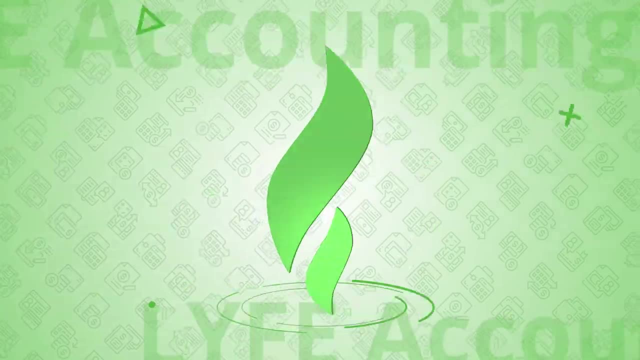 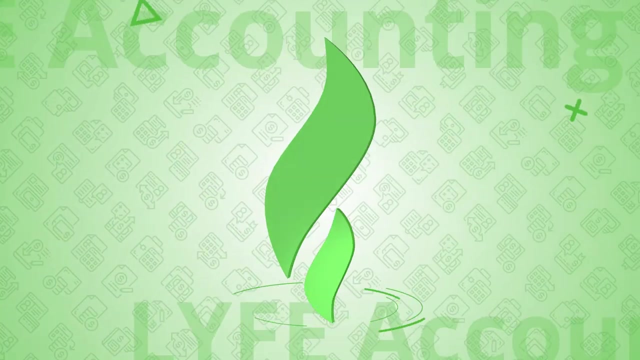 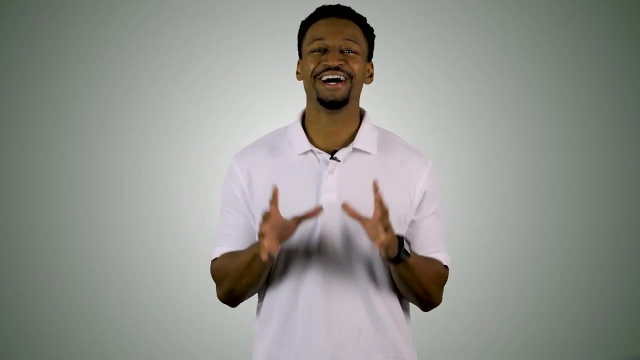 your current pay structure, then this video is for you. Hey guys, I'm Sean with Life Accounting, the accounting firm that saves businesses from high taxes and low profits. Now, I know a lot of you guys out there, especially if you're in the early. 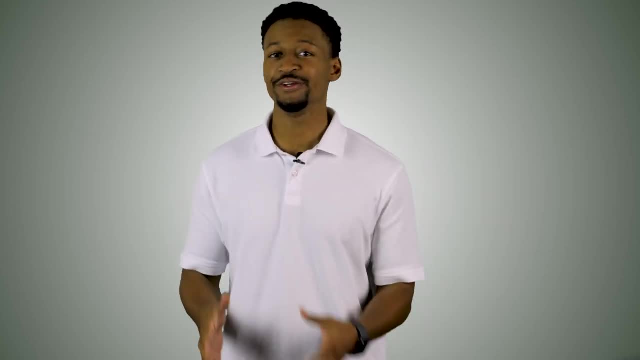 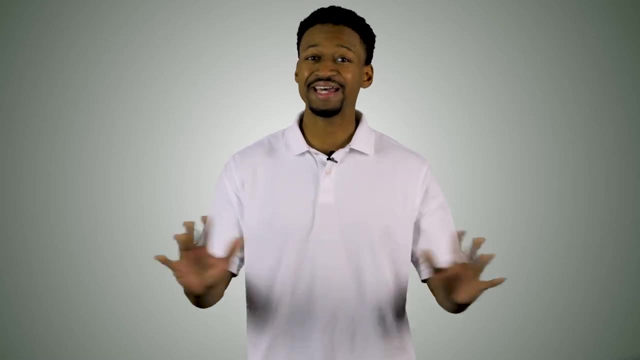 stages of starting your business, are wondering how you should pay your first employee, Which, if you're at this point, that likely means that your business is growing or is proven, which is not an easy feat to accomplish. So I just want to take a moment to congratulate you on all your growth so far. 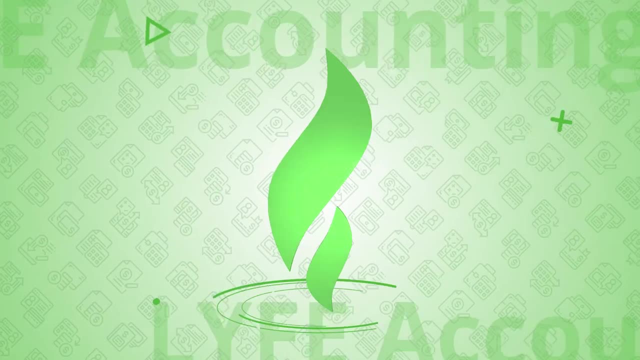 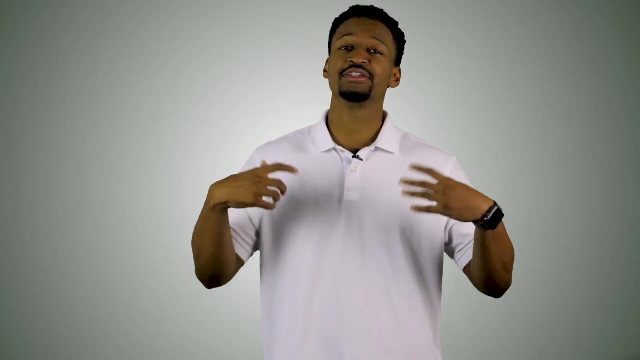 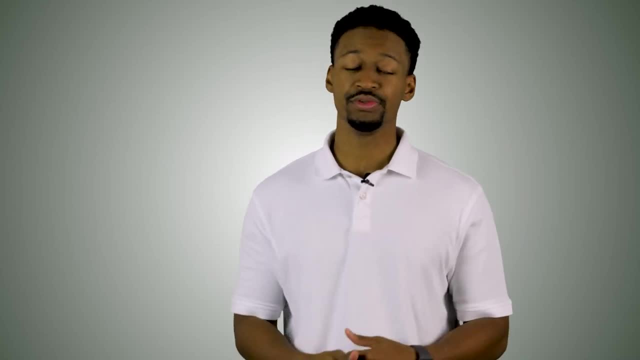 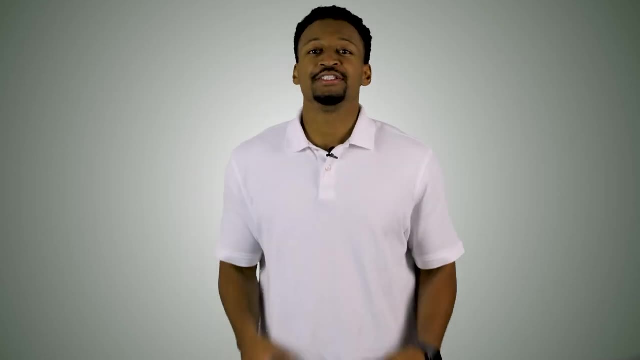 Number one reason why people would even consider working with you. And, as we know, business is tough, so you want to be as competitive as possible so you can attract good talent. So we want to maximize our pay structure between contractors and employees so we get the best. 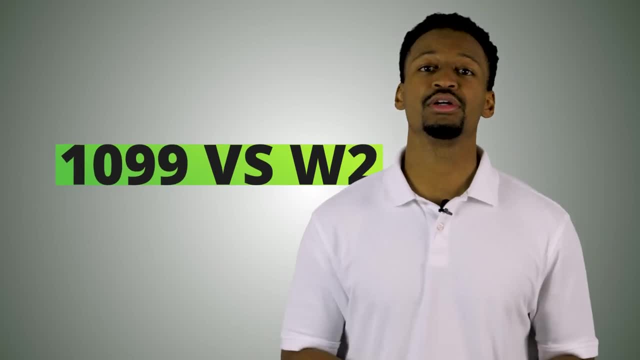 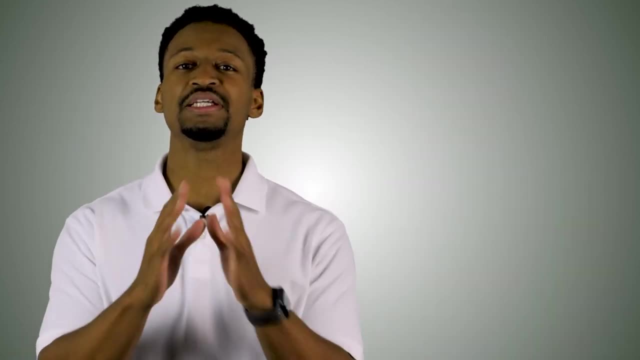 outcomes for everybody. So today, in this video, we're going to discuss 1099s versus W2s, and which one may be better for your business. But before I dive in, please do us a huge favor by subscribing to our channel and liking our 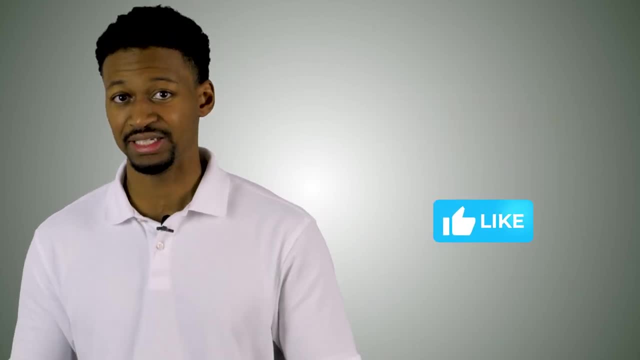 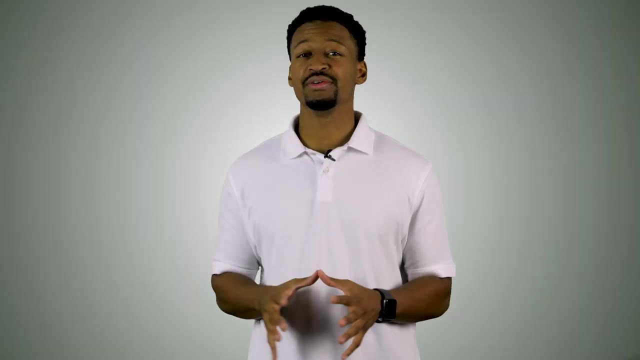 video so we can continue to bring you valuable content. We interrupt this broadcast to bring you a special. please subscribe alert. Thanks in advance. Okay, so here's what we're going to cover in this video Number one: we're going to define what a 1099 worker is and what a W2 worker. 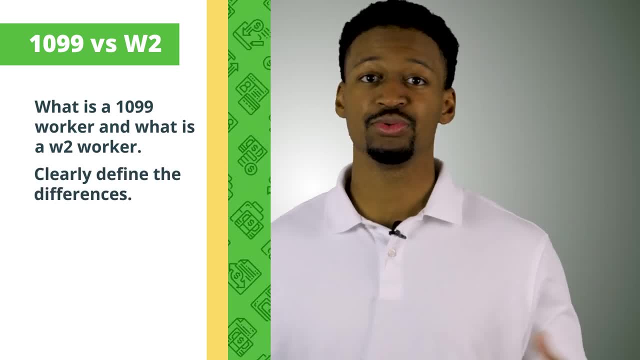 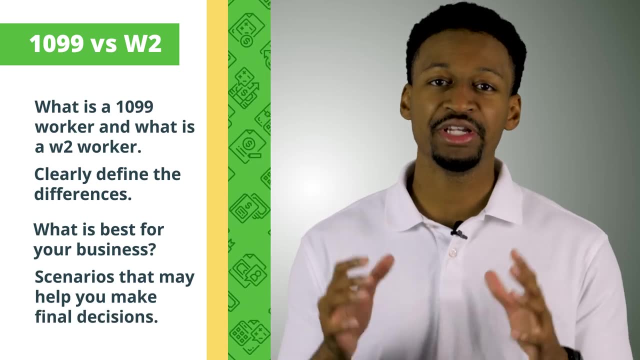 is Number two, we're going to clearly define the differences between a 1099 worker and a W2 worker. Number three, we're going to look at what is best for your business. And number four, we're going to make sure we understand everything by looking at some real examples. 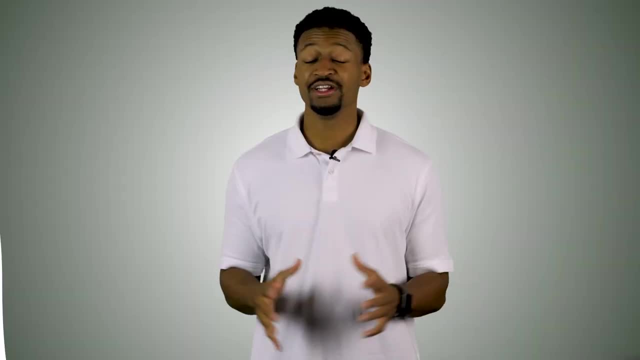 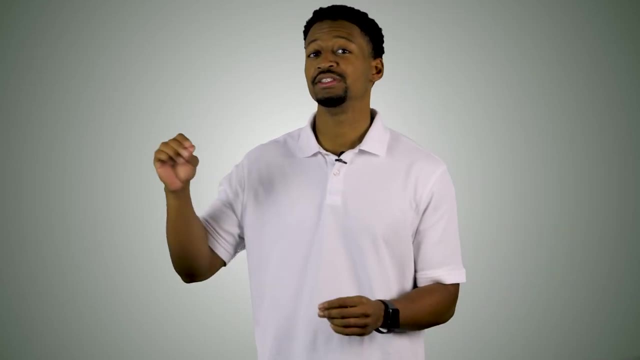 and may help you make a final decision. All right, now that we got that out the way, let's go ahead and dive in by defining what is a 1099 worker and what is a W2 worker. Let's start with a 1099. 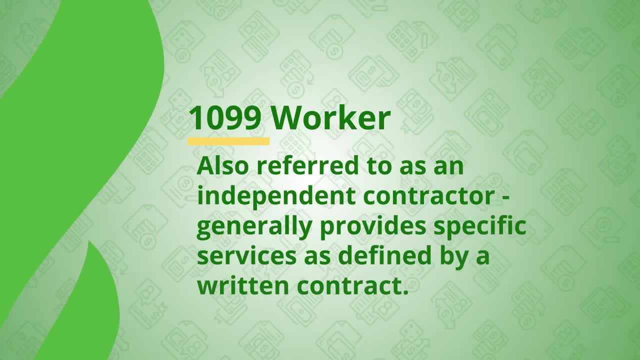 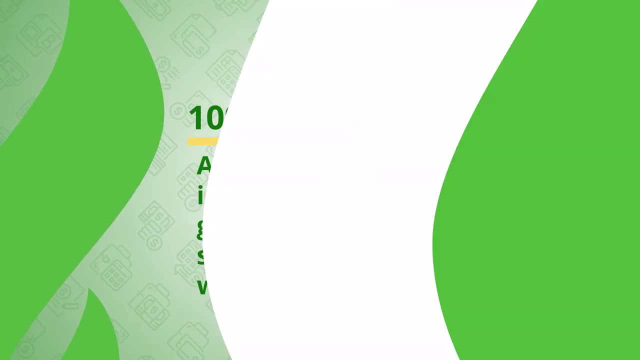 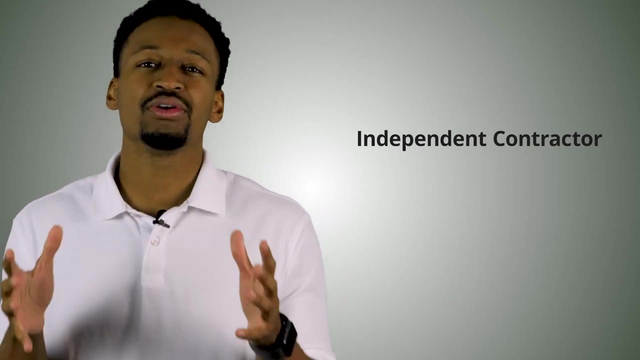 worker, So a 1099 worker, which is often referred to as an independent contractor, generally provide specific services with a well defined written contract. So freelancers and consultants are often declared as independent contractors and thus are self-employed employed, so these are business owners themselves who likely work with multiple clients independent. 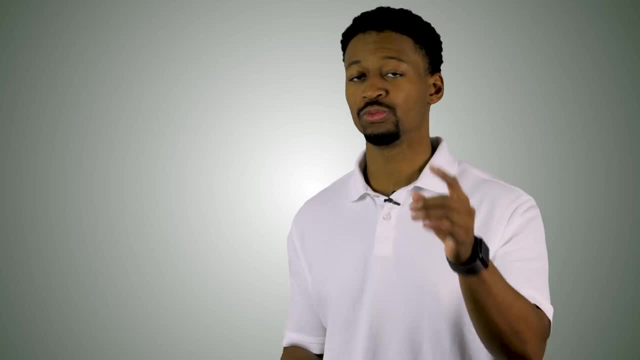 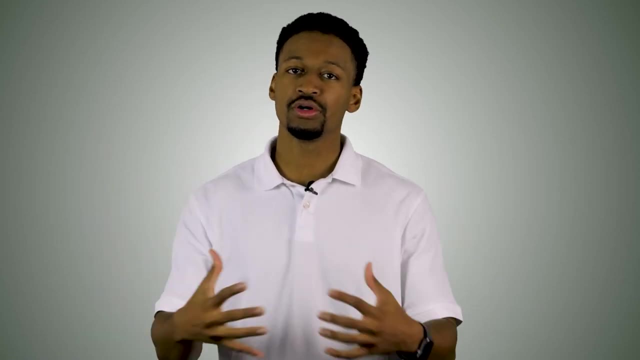 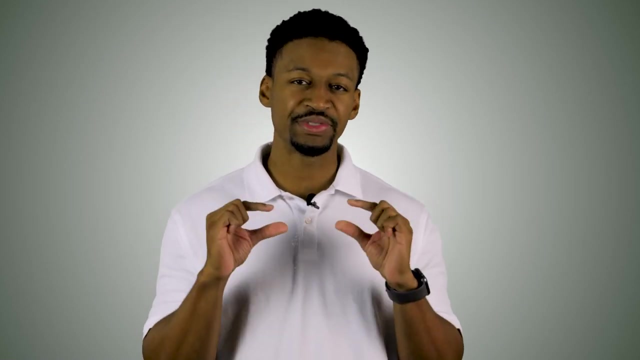 contractors have complete control on how they work with you. so, as an independent contractor, if you want to hire a team, then you could. so you basically control all your own profits and all your own expenses. now, usually, a business will engage with an independent contractor for a very specific 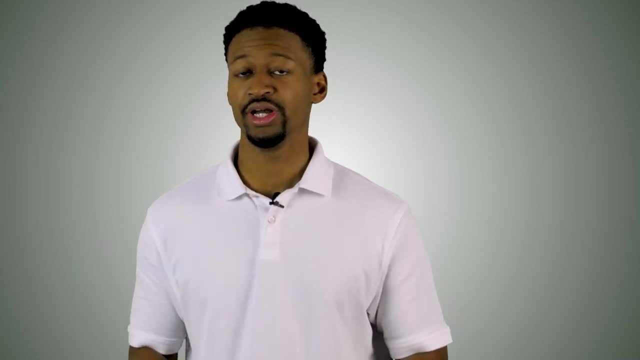 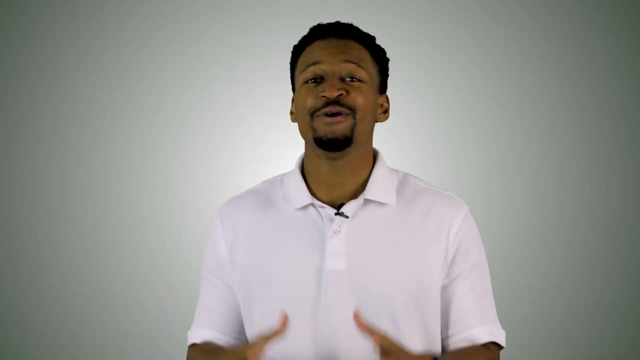 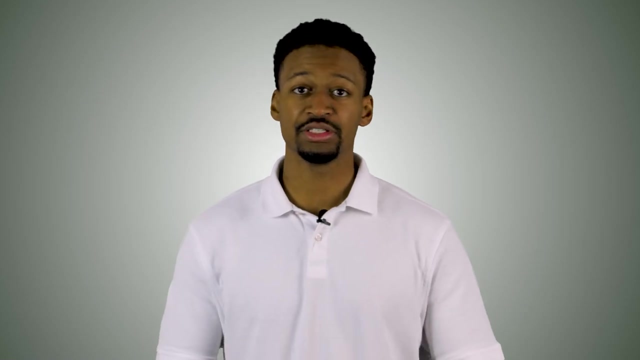 period of time with, again, a specific contract, but that engagement can be renewed as many times as that independent contractor in the business would like. now, when you work with an independent contractor, your level of control is relatively low, so your level of financial and legal responsibility is also low. you don't have to pay payroll taxes or benefits or a lot of other things. that you might have to do with a w-2 worker, like health insurance, pto or even overtime. so by hiring contractor you're able to save some money, but you lose some flexibility because you have to stick to the agreement or contract that you have in place. now let's move on to define what exactly is a w-2 worker. so w-2 employee. 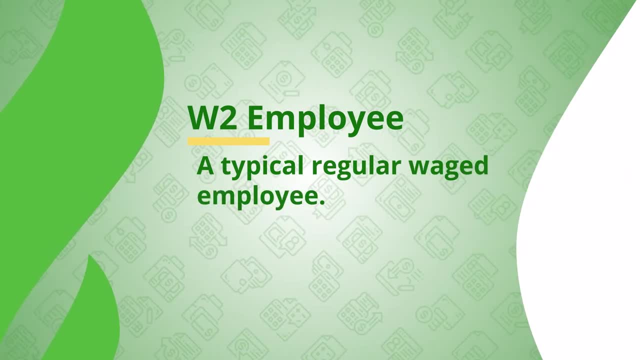 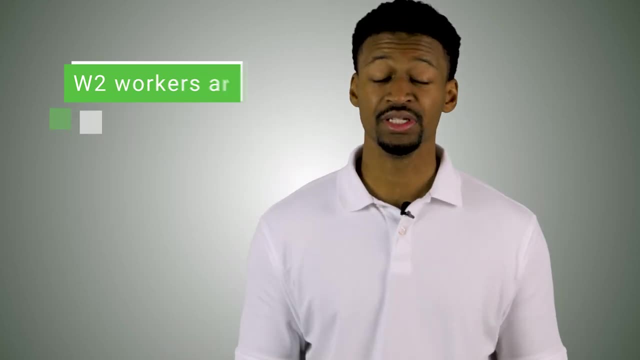 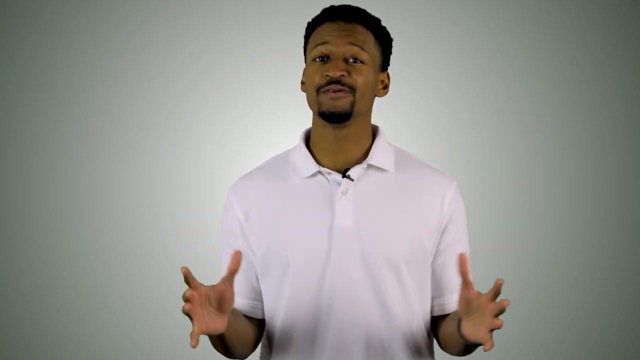 is what we'd like to think of as your regular wage employees. unlike independent contractors, w-2 workers are not business owners. they work solely for your company, so you have their full attention, and so you have to take care of them a little bit more so w-2 workers can participate in all your employee benefit programs and work according to your current business needs and schedule if you're not happy with their performance on the job, and most states will allow you to terminate the relationship immediately, whereas with an independent contractor, you're expected to uphold the agreement for a very specific period of time. so you gain a tremendous amount of flexibility by 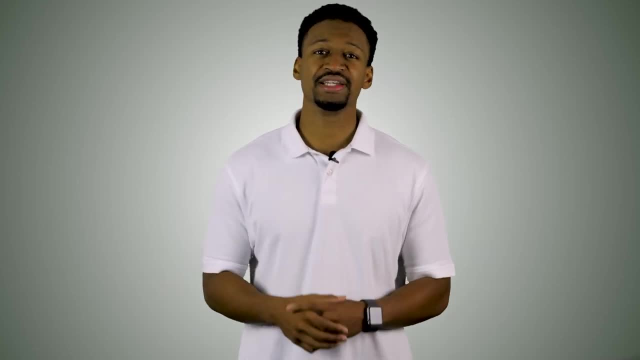 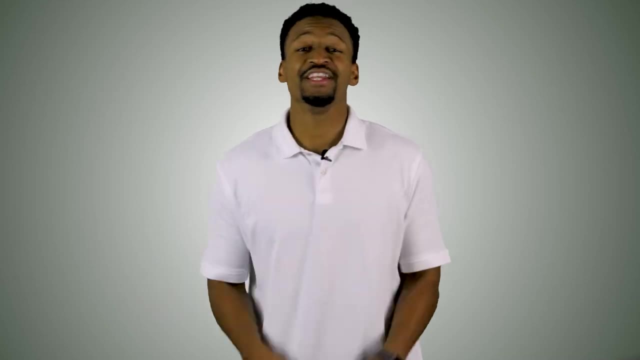 hiring a w-2 employee and unless you classify your worker as an independent contractor, then the D D fault classification for someone working for your business is a w-2 employee. now there are some laws and regulations for w-2 employees. firstly, and of course you 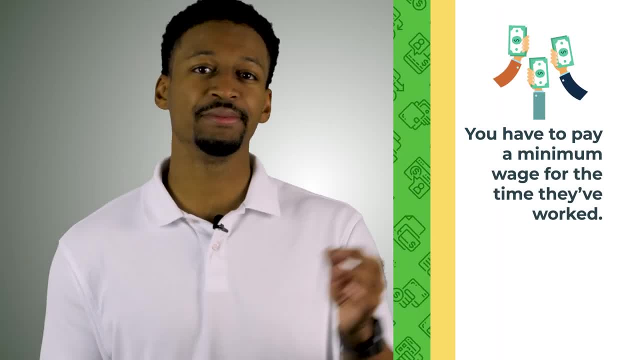 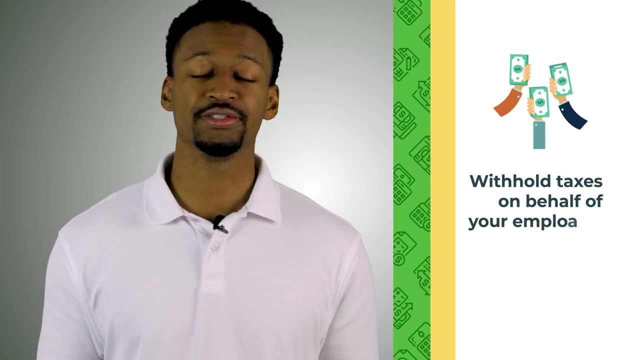 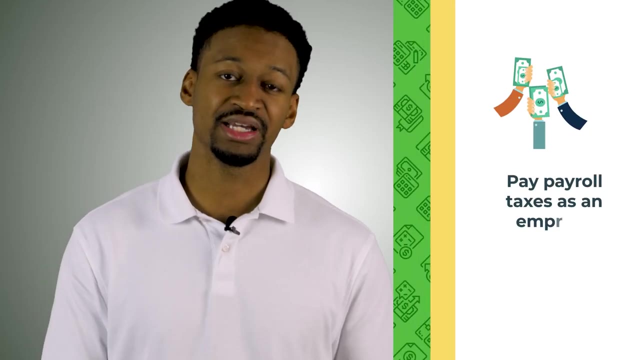 have to make sure you're paying your employees a minimum wage for the time that they work, which that minimum wage is often set by the state and federal laws. also, you're expected to withhold taxes on behalf of your employee, such as Social Security and Medicare taxes. also, you're expected to pay payroll taxes, as 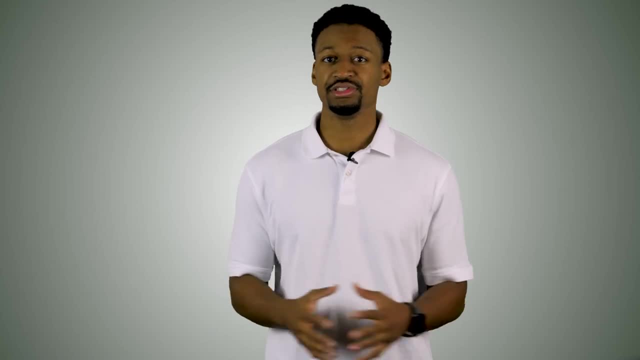 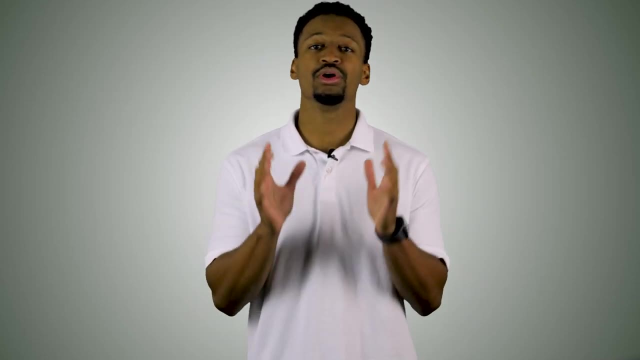 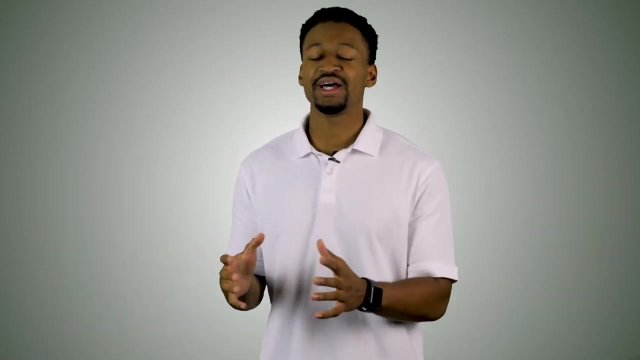 an employer and, as we mentioned earlier, benefits such as health insurance, retirement contributions, paid time off, can also be other incurred expenses, whereas with an independent contractor, they're expected to handle all their benefits on their own and since this is the case, you may find that independent contractors are. 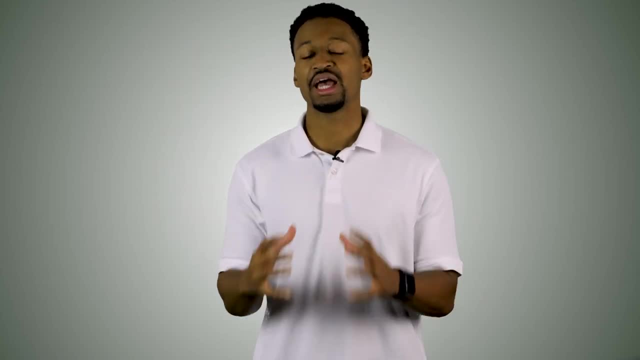 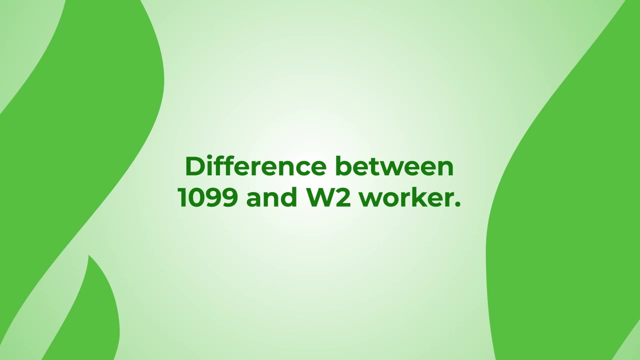 charging a premium rate or a fixed fee to account for some of those other expenses. okay, now let's move on to section two of this video, where we get a little bit more specific and determine the difference between a 1099 versus w-2 worker. now both are named after their respective tax forms: companies. 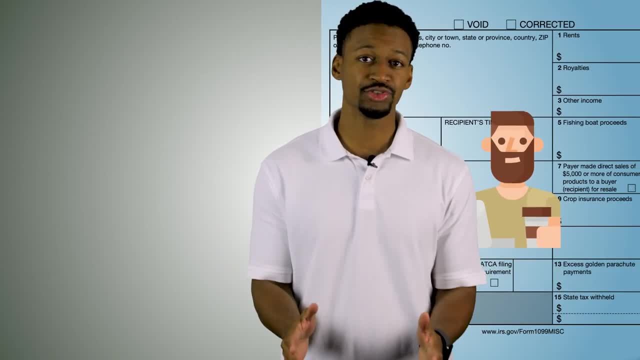 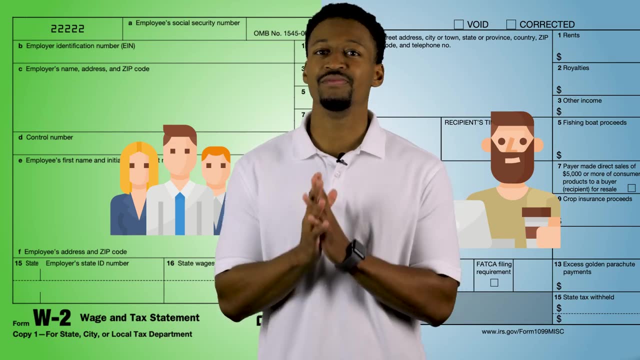 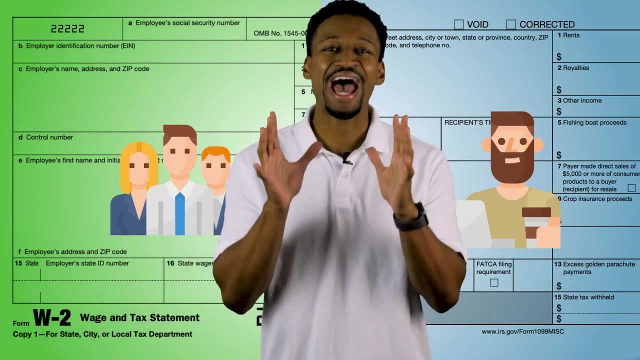 provide a 1099 miscellaneous to independent contractors, and companies file a form w-2 on behalf of their employees and, as we know, having the right workers are vital to your success as a small business. so the question isn't: should we hire workers? the question is: how should we classify them? 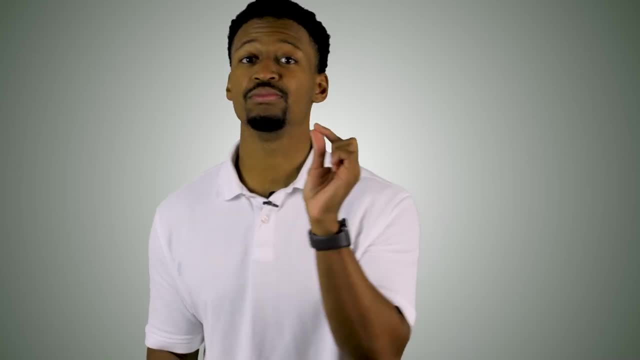 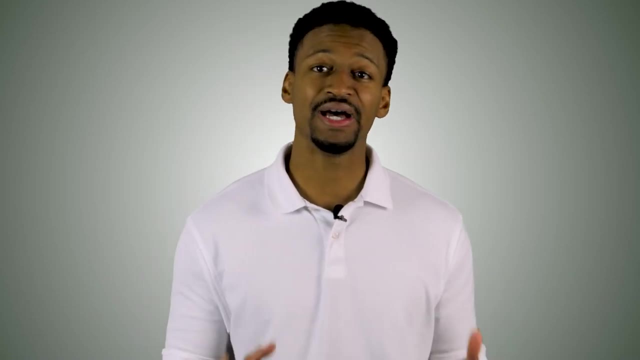 and it is very important to classify them correctly, because if you misclassify an employee as an independent contractor, you're not going to have to contractor, for example, and you can be subject to thousands and thousands and fines and legal fees. and i want to help you cut down on some of the confusion and help you with how to classify your. 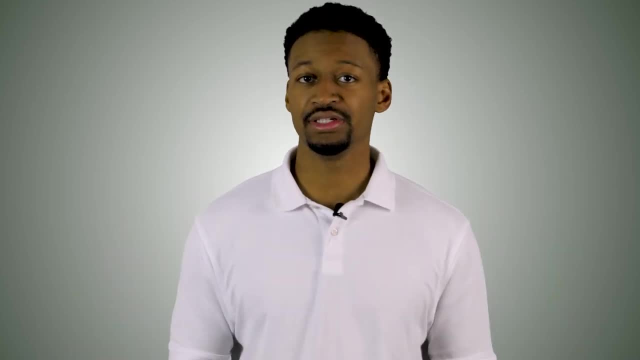 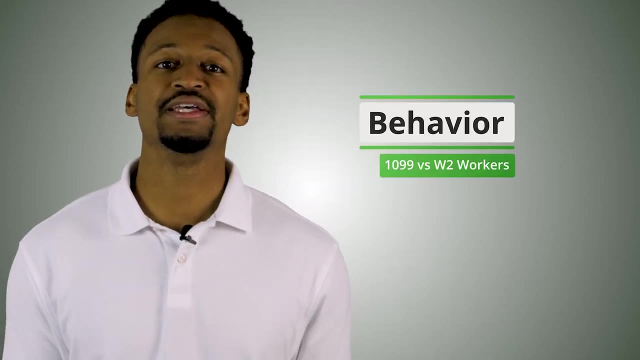 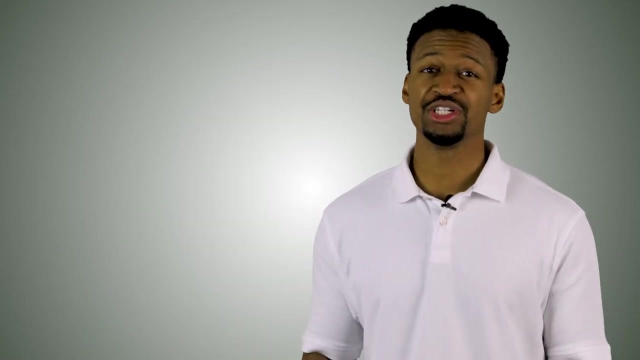 employees. so we're going to look at exactly how the irs does it, and they look at these three major categories when determining 1099 versus w-2. the first category is about behavior. so basically, the irs looks at the relationship between the company and the worker. you should ask yourself a question. 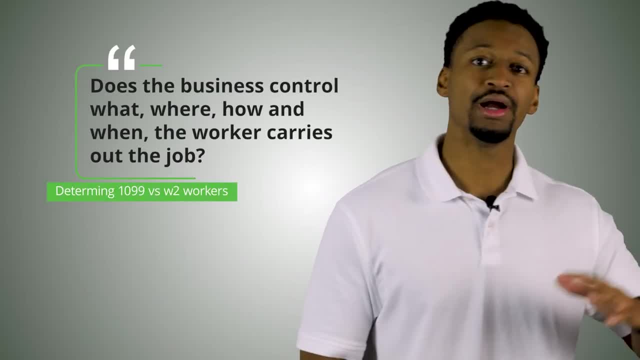 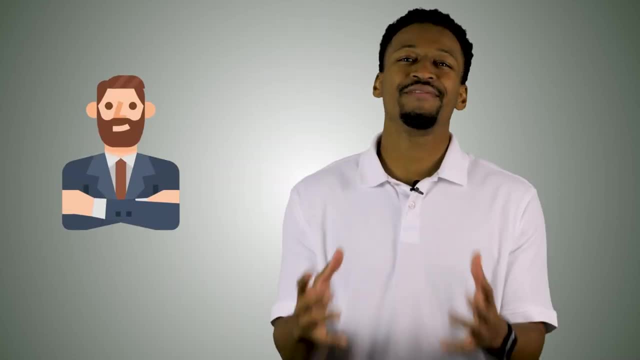 like, does the business have control over what, where, how, when the worker carries out the job, and so the more control that you have, the more flexibility you have, and then that fits closer into the w-2 category. now, the next category that the irs looks at is the financial relationship. so 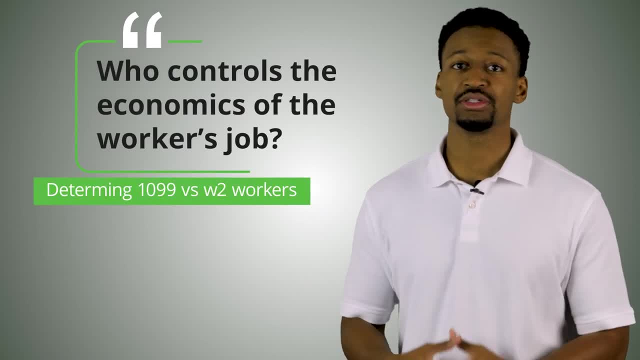 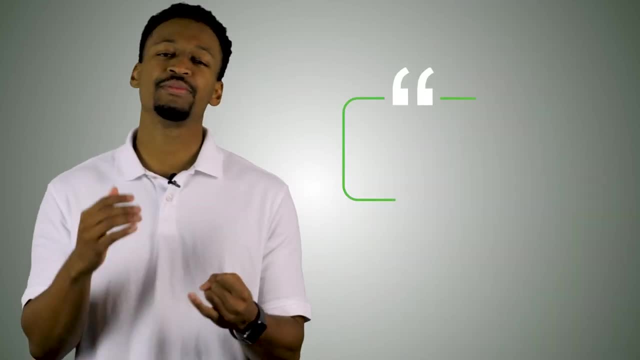 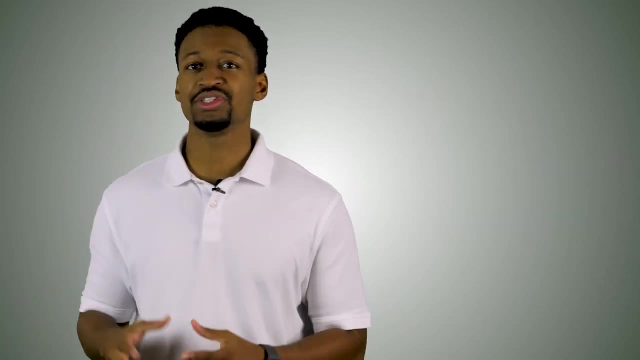 the question you want to ask here is: who controls the economics of the worker's job right like: are you setting the salary or is the worker explaining their fees to you? also, what's the payment method? is it hourly? is it hourly or is it more of a fixed fee? so in a financial relationship, if the worker is setting, 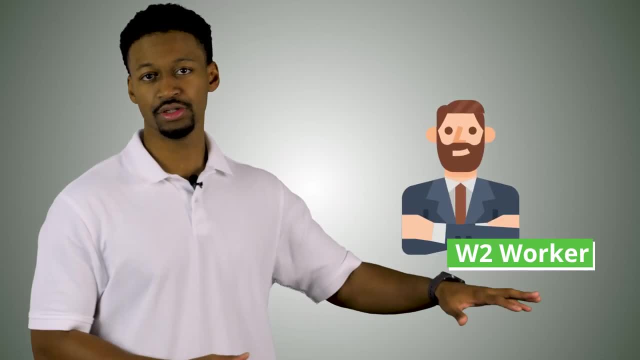 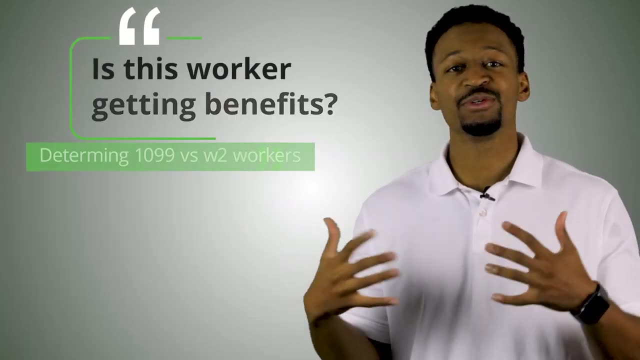 more of the fees. then it's closer to an independent contractor relationship and the last thing the irs will look at is the overall type of relationship. so they'll ask questions like: is the worker getting any benefits? are they working for a specific period of time? is there a very strict agreement? 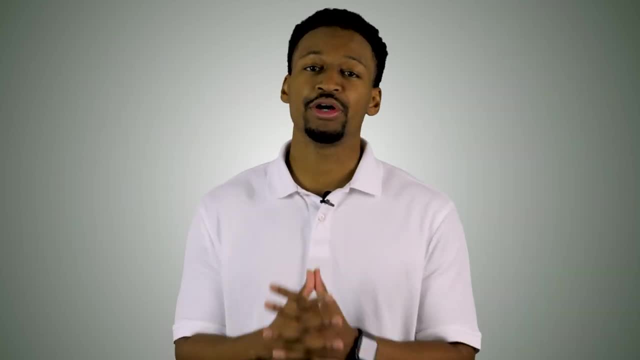 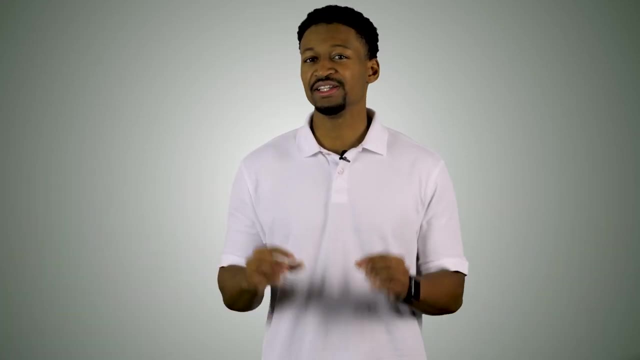 in place between the employer and the worker. these type of questions will help you and the irs determine the relationship between your business and the employees. so what it all really boils down to is the level of control that a business has over the worker. if the worker has a lot of independence with little oversight, then they're 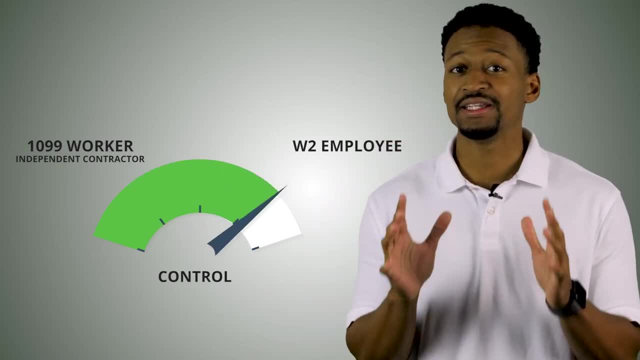 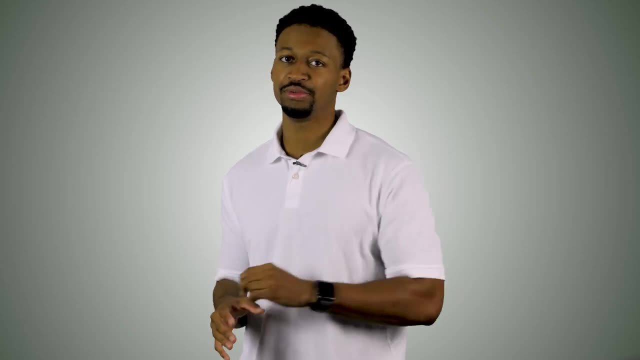 more likely an independent contractor. if the business has a lot of control, then they're more likely working with a w-2 employee. so that's exactly how you want to go about classifying your people. now, if you're still unsure about how to classify your employees, then you can file a. 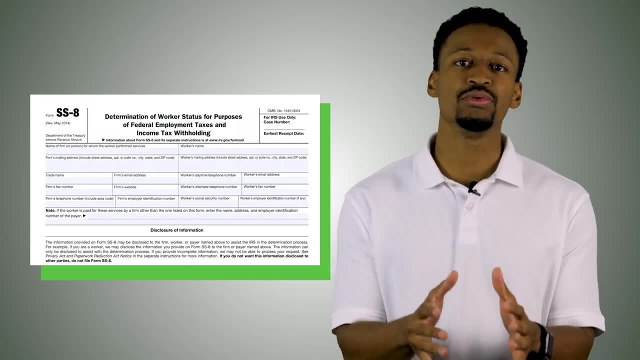 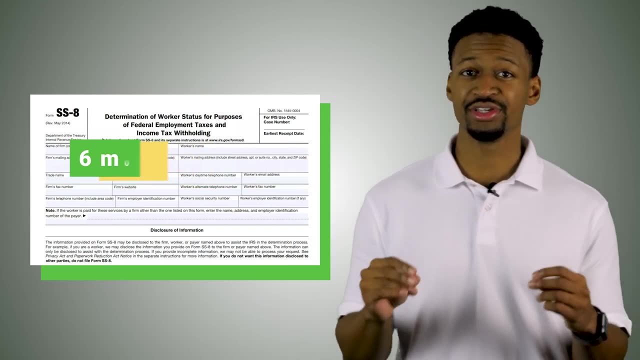 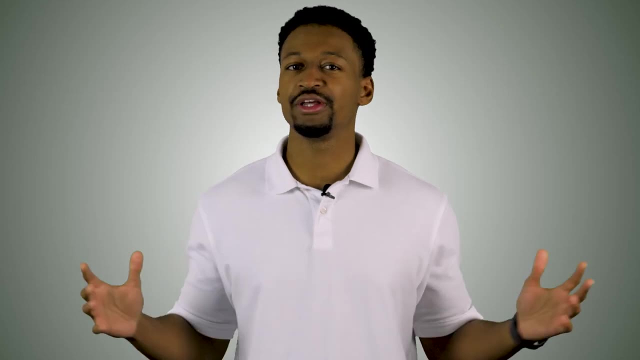 form called ss-8, and the irs will help you with this classification, but it can take six months to get to the point where you can get the answers you need as quickly as possible. okay, so now that you understand the differences, let's go ahead and talk about the question. you've probably already been asking yourself which is number three on our list. between a 1099 versus employee, which one is best for your business? so, of course, as a small business, costs are really, really important and employees are going to have a higher cost. you have to pay employment taxes, worker compensation office. benefits. you have to have a higher income and you can quickly eat away at your profits, so most people will try to start out by hiring independent contractors. however, you have to factor in the opportunity cost, because that can level the playing field between 1099 versus w-2 workers. 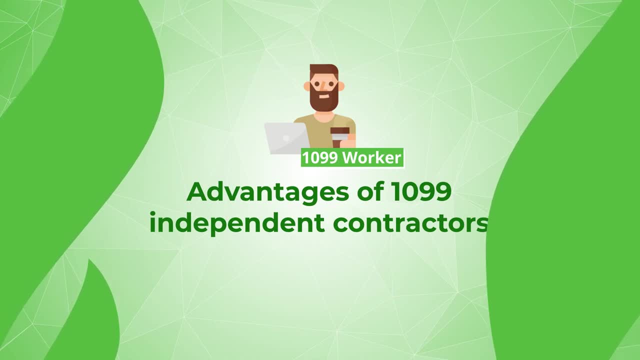 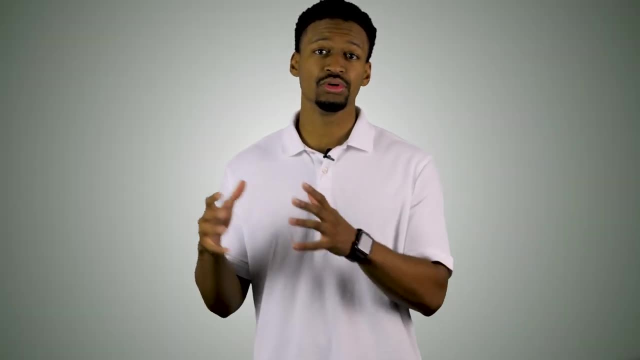 so let's go ahead and look at my top advantages of hiring a 1099 independent contractor. number one: they can bring some specialized experience. the biggest benefit of working with an independent contractor or a business is they normally focus on one or two areas of their business and they're 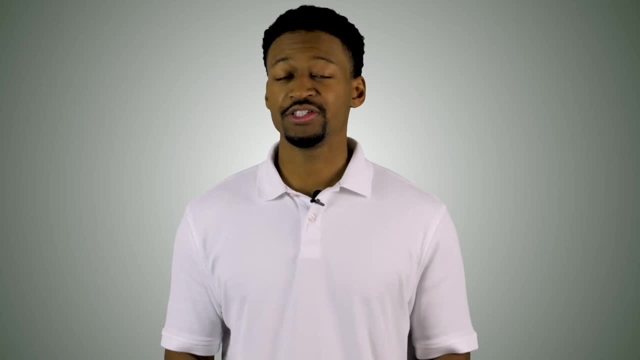 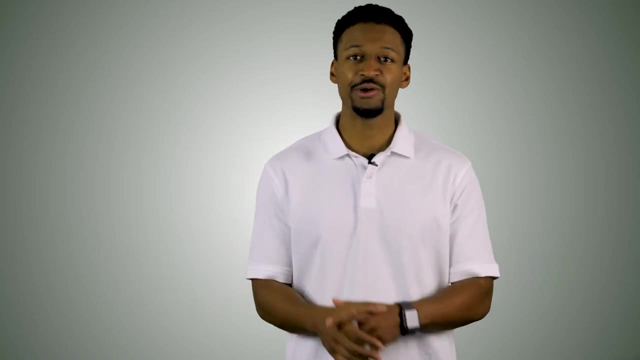 really good at it. so if you have a specific project that is short term, then they can be great for you, for example, if you're moving into a new office and you need some help with a layout and design, and hiring an independent project manager would be a good idea. number two: you have more budget. flexibility. so, instead of hiring somebody that you have to pay for the long haul, you can set a predefined budget and outcomes so that you are being as cost efficient as possible. number three: they come with less legal risk, so they're going to be more flexible and they're going to be more. 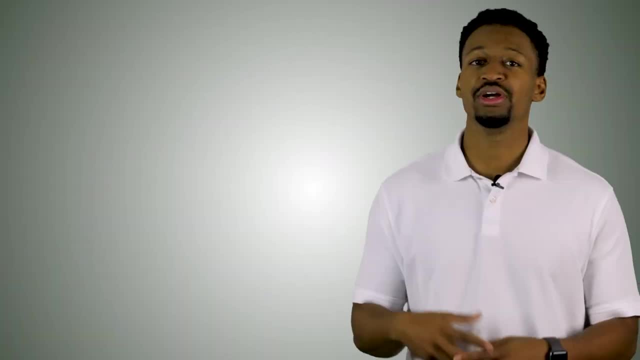 flexible and they're going to be more flexible and they're going to be more flexible. so when you have a w-2 employee, you have to get workers compensation, whereas with independent contractors you don't. in fact, most of the time independent contractors come with their own insurance. 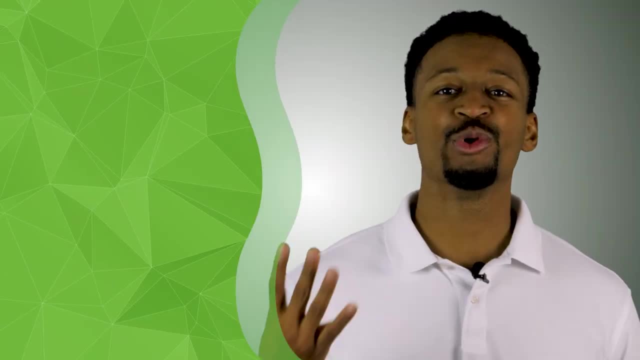 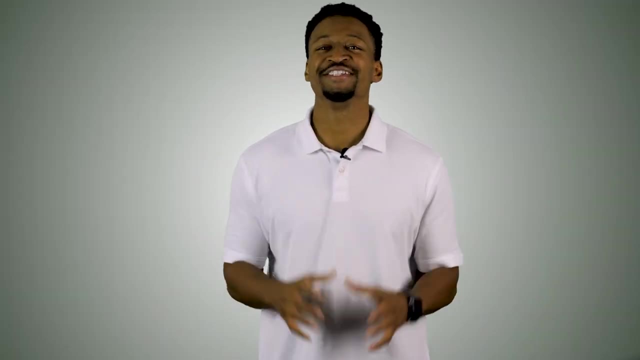 that limits your risk to legal exposure. number four: you have a lower volume of administrative work so, as we mentioned, you don't have as many laws that come with a w-2 worker, so you don't have to worry about calculating employment taxes or putting together big benefit plans. 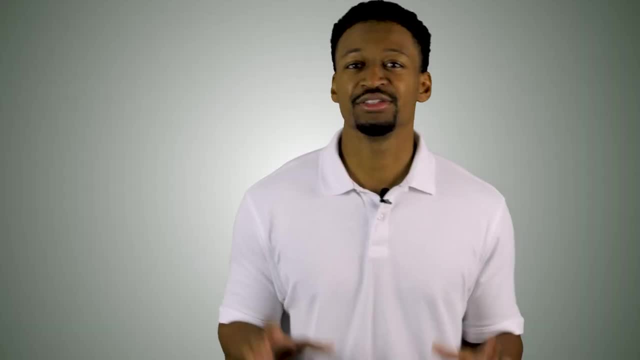 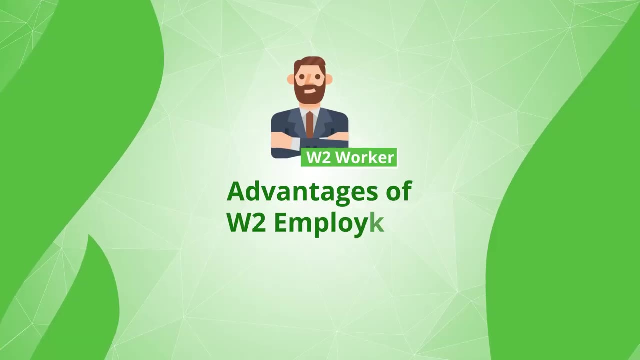 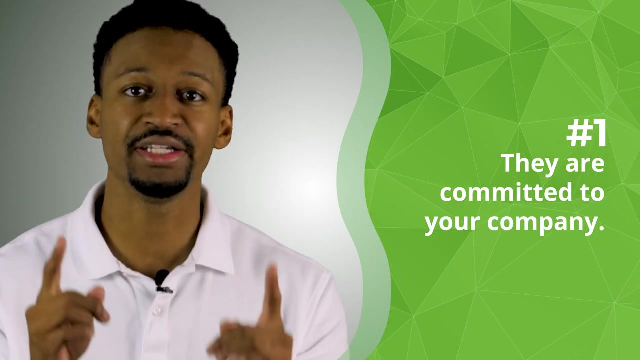 or just making sure that everything is administered correctly. so those are some of my major benefits when it comes to independent contractors. sounds pretty good, right? well, hold on, because w-2 employees have four great benefits, and you should factor in as well. number one, the first advantage, and probably my favorite, is that they're committed to your company. 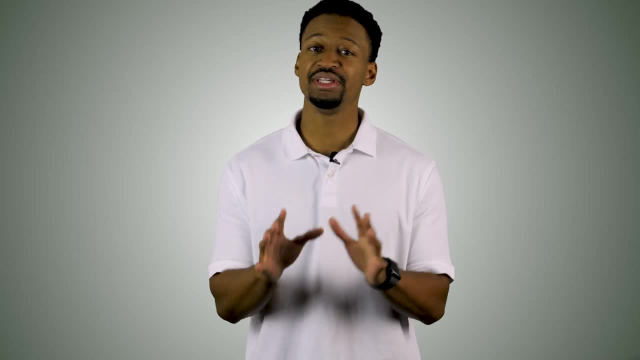 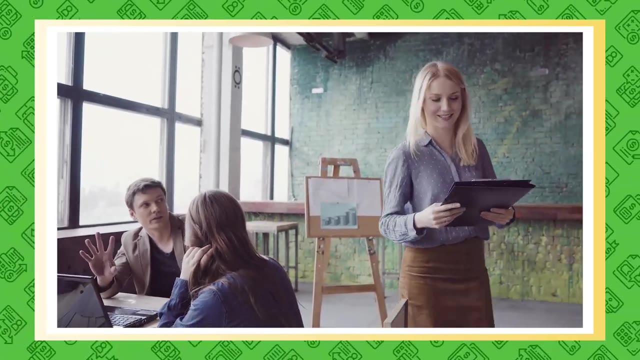 and when you have a great culture, your employees can thrive beyond just their job description. they can take on your vision and really work as an extension of your goals and your aspirations, and the performance is very clear and measurable. you never have to worry about if they're going. 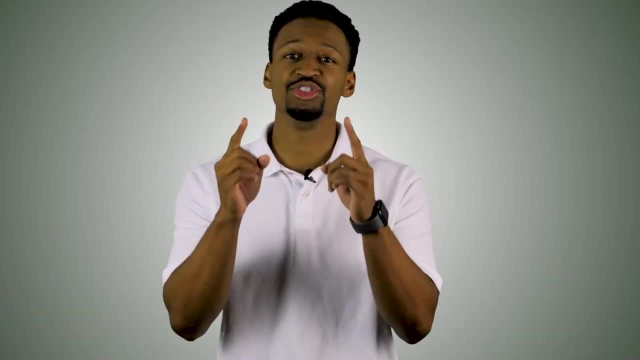 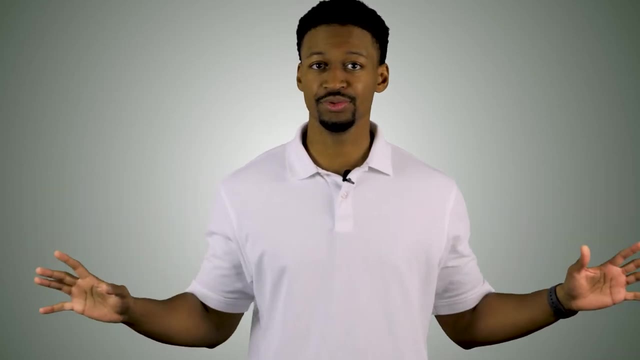 to go to work today or if they're even going to respond to you because you set the schedule now. there are some great independent contractors out there as well, but you may just be one of many clients for them. number two: another great benefit is that w-2 employees offers more. 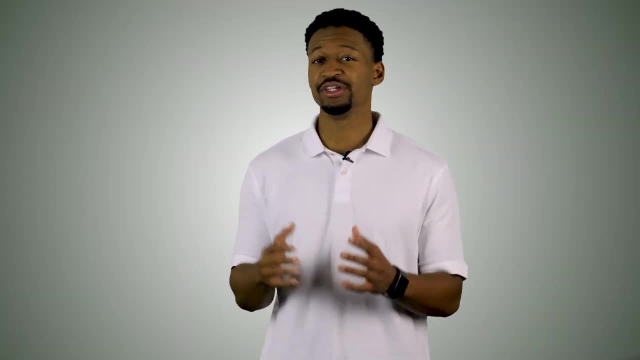 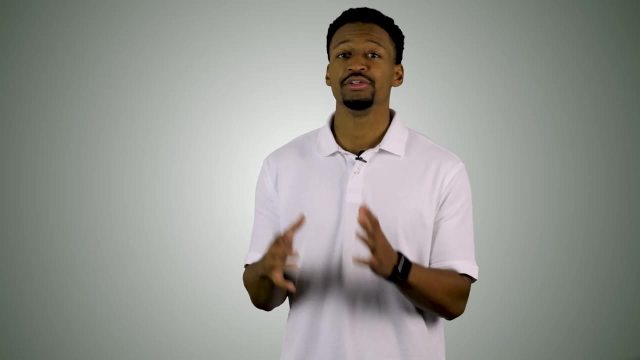 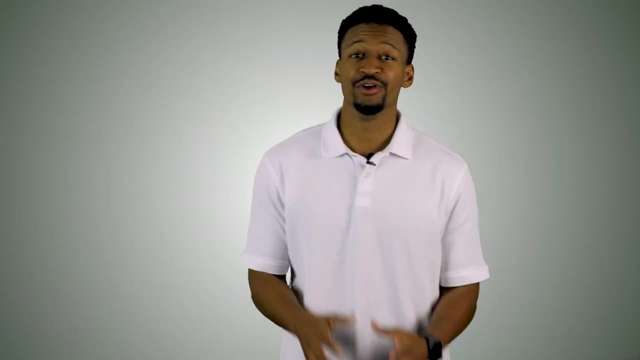 continuity, because working with an independent contractor can be a short-term relationship when you have to hire a new one and you likely have to re-explain what your company is, what you do, your brand and your overall vision again and again, and again and again, whereas a w-2 employee can easily shift between projects because they have 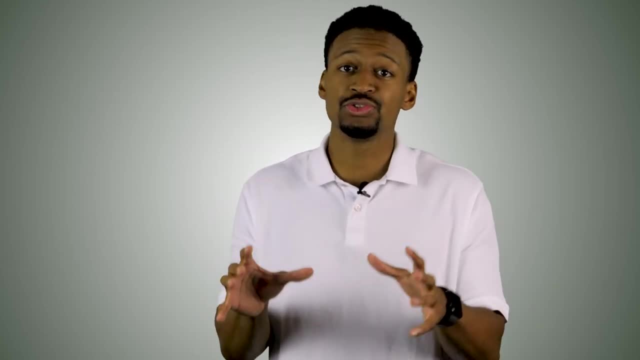 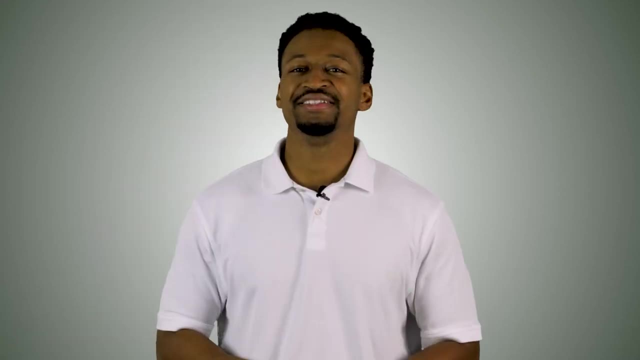 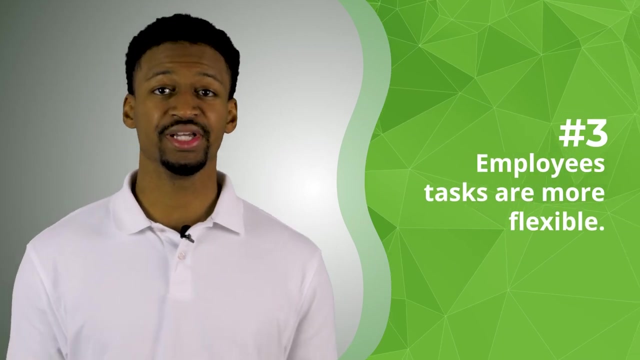 a long-term relationship with you and they naturally understand the business. so this ultimately saves you a lot of hours and just re-explaining what your business does, not to mention the other hundreds of small details that often get missed. number three: employees. tasks are more flexible. usually independent contractors are good at one or two things, but when you're running, 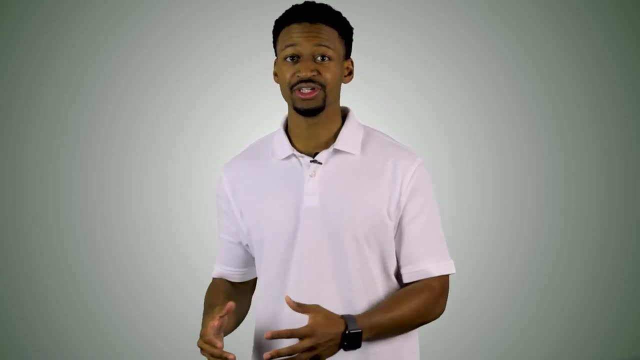 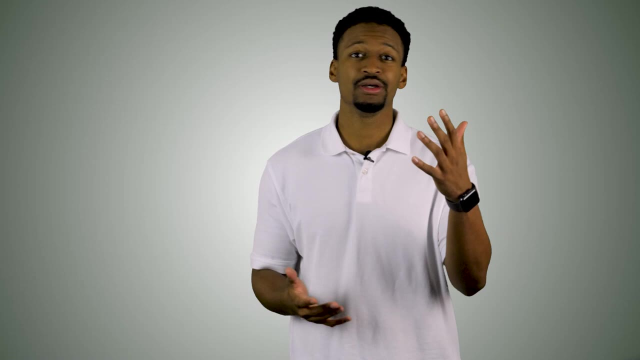 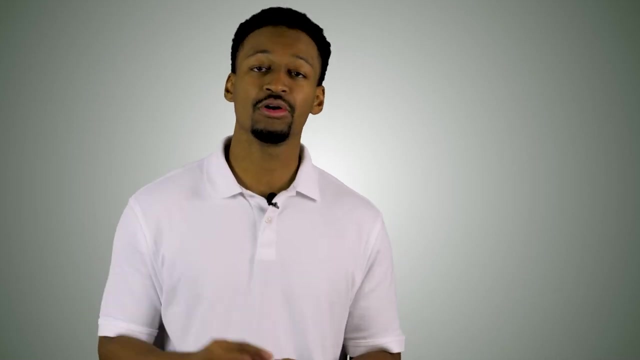 a business. especially when you're running a business, you're going to need a few hours to get to the point that is growing, and there are hundreds of other tasks like answering phones, training other people, customer service, billing, collections and a lot more. so the advantage of having employees is that they can help you out with some of these. 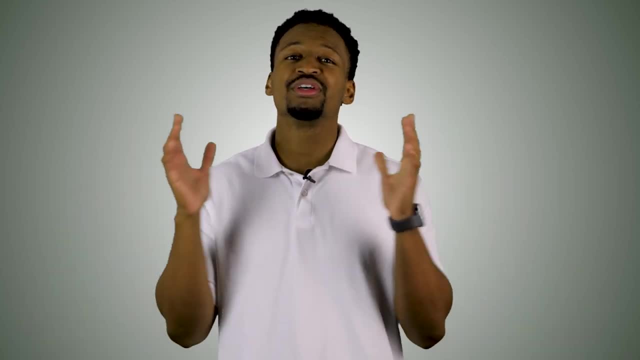 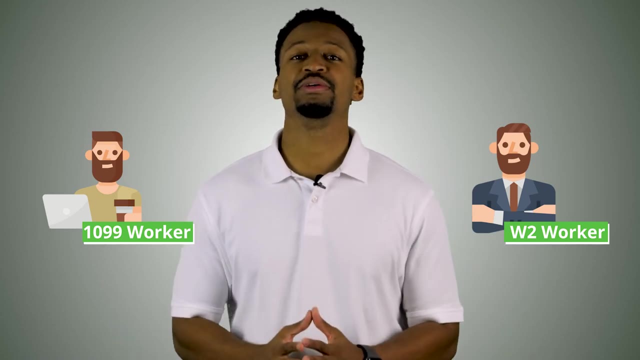 small but very important things that need to get done. so, overall, no one can really say whether an independent contractor or w-2 is better than the other. it really just depends on your budget, your timeline and the level of control that you have to make, and then, of course, this is also important. for you to understand that you're going to need to be in a position to be able to act on the other tasks that you've done. so if you're looking for a small and important task, why don't you go to one of your employees and try to get that done, or try to get it done, and you can do it at the end of the day. 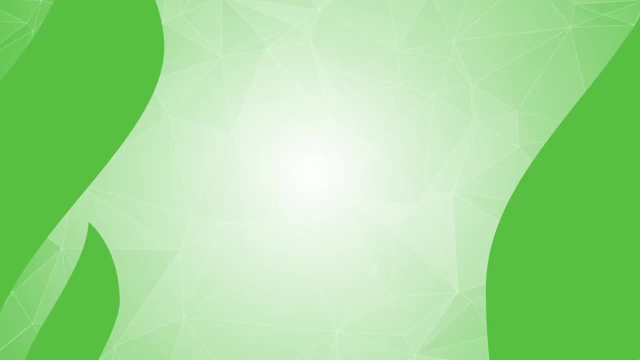 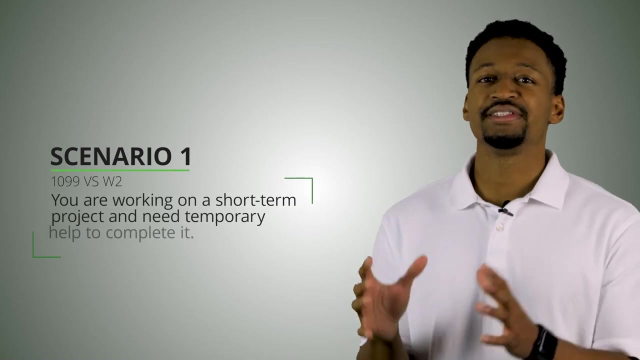 that you need. All right, let's look at the last section, section number four, where we go over specific scenarios for a W-2 versus 1099 worker. Here's the first scenario. Let's say you're working on a short-term project and you need help to complete it temporarily. Should you hire a 1099? 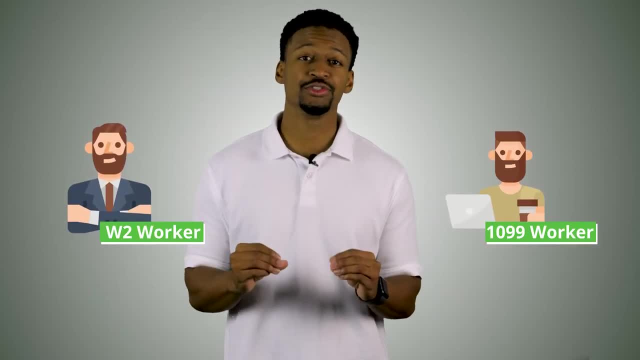 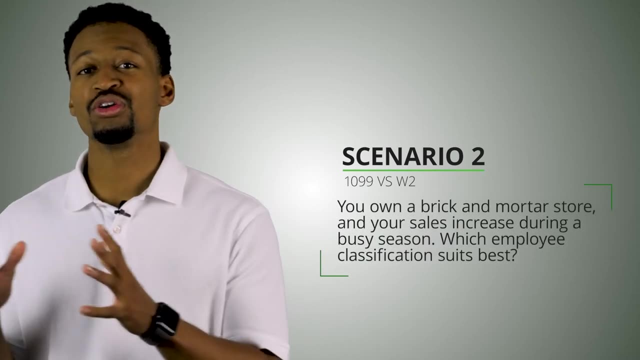 or W-2 employee. Well, since this is a short-term contract, an independent contractor would likely be best suited to handle this project for you. All right, how about this scenario? You own a brick-and-mortar store and your sales go through the roof during a busy season. Which employee? 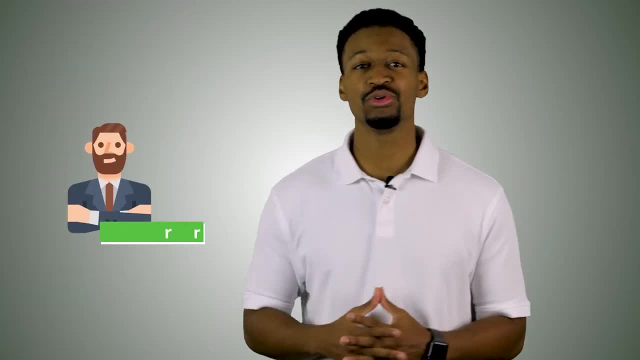 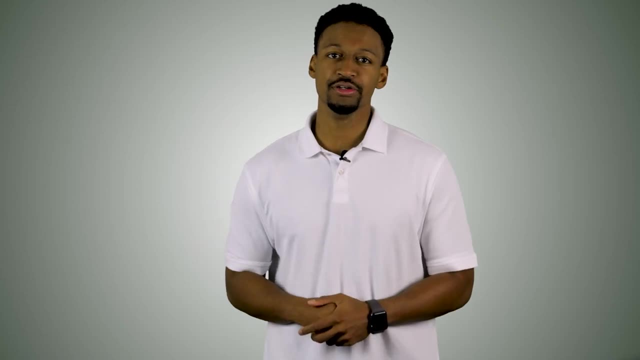 classification suits best. In this case, a W-2 employee fits best because you need someone who can be on a very specific schedule that can be adjusted. All right, what about this third scenario? There's a function in your business, like taxes or bookkeeping, that needs to be taken. 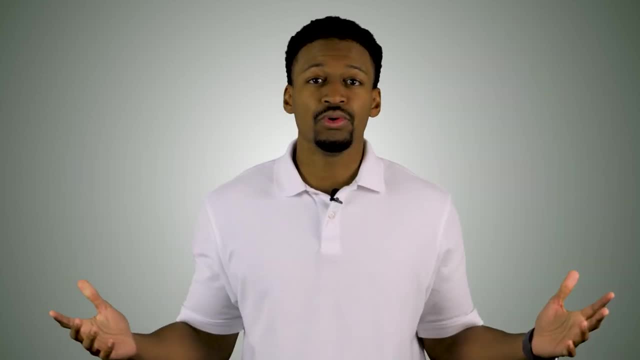 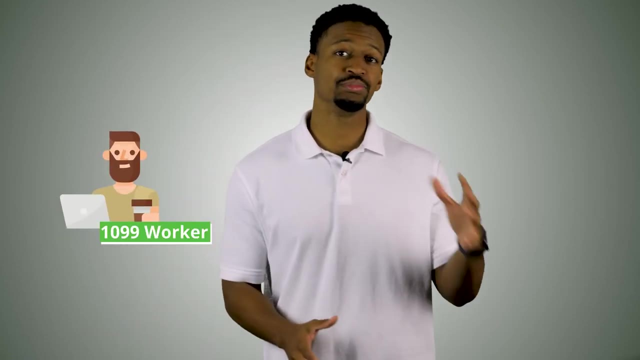 care of regularly and only takes a few hours. Now, this could go both ways, but if you don't have enough hours for this task for someone full-time and you likely should hire an independent contractor, regardless of the situation, then you should hire a W-2 employee. All right, let's look at the 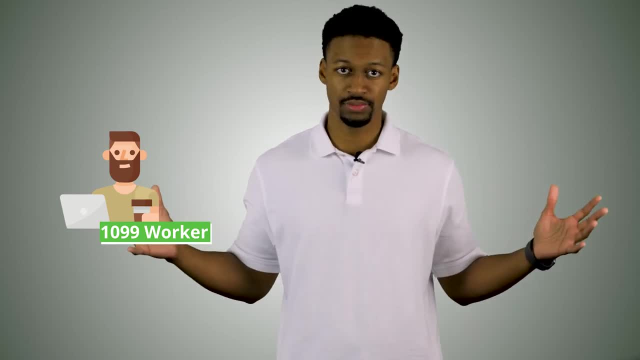 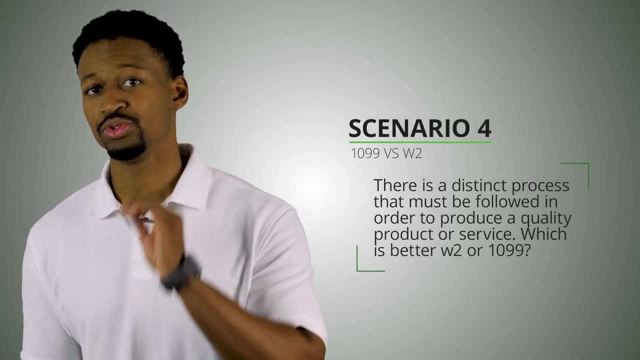 business instead of paying for someone full-time or long-term. All right. last scenario, and I'm going to give this one to you guys, Let's say that there's a distinct process that you must follow in order to produce a quality product or service. Which one is better, W-2 or 1099??